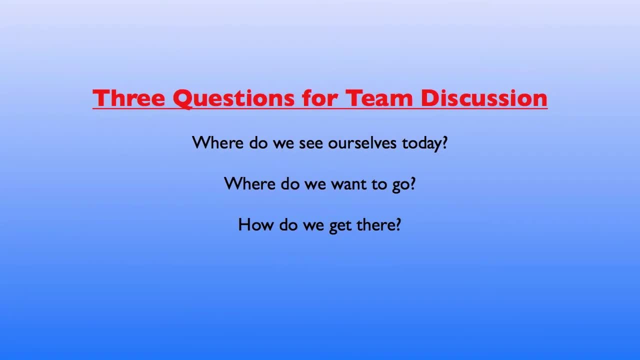 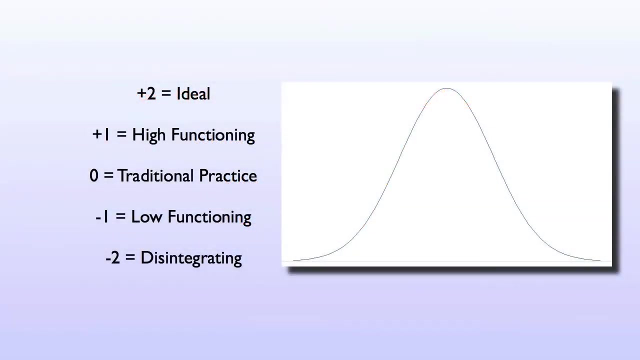 goal in mind. I would call that goal consensus by the leader and members of a team on the answers to three key questions regarding team trust: Where do we see ourselves today, Where do we want to go And how do we get there? I like to use the image of a bell curve from. 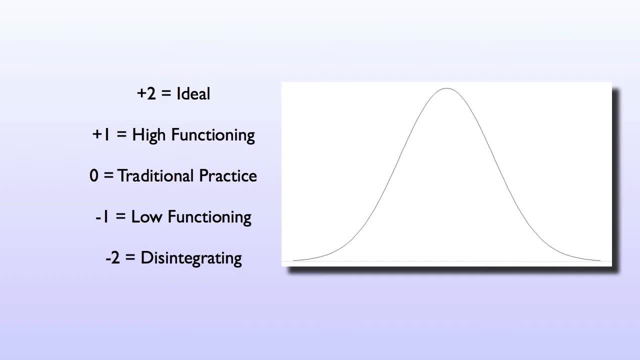 the field of statistics. to begin talking about levels of team trust, I want you to understand that a bell curve is more a metaphor than a scientific analysis, but it also can be quite helpful to visualizing the continuum of levels Most teams are in the middle of. 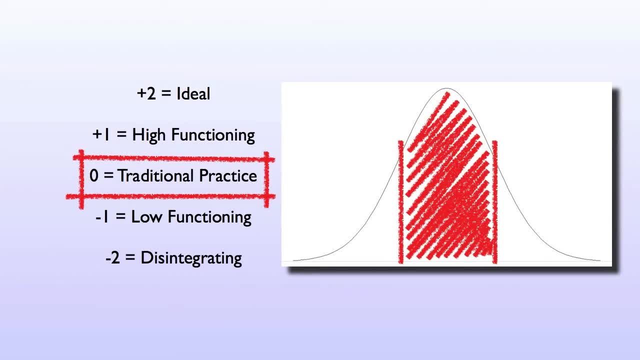 the bell curve somewhere between low and high trust. They are governed by the conventions of traditional workplace culture, a culture for most organizations that has its roots in hierarchy and an ethic of individualism. People tend to get their work done and the team performs. The focus is usually on getting the tasks and projects completed on time. in 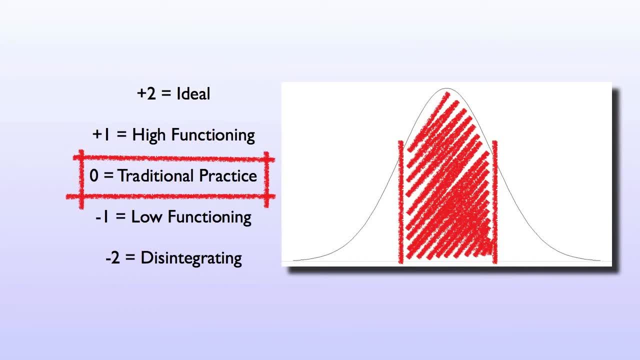 budget and with a minimum of errors. Often there's a manager or leader who keeps the team on track, handling performance issues or interpersonal problems and disputes in the background. I'd emphasize: there is nothing wrong with this team, but it has unexamined 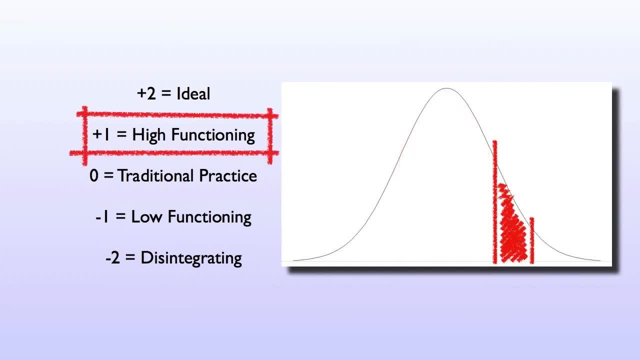 and therefore unexplored potential. When teams move to the plus one high functioning level, things begin to change, largely because of a conscious and intentional team decision to help the group be all that it can be. In plus one teams, people learn to take risks, to speak up with one another and to address 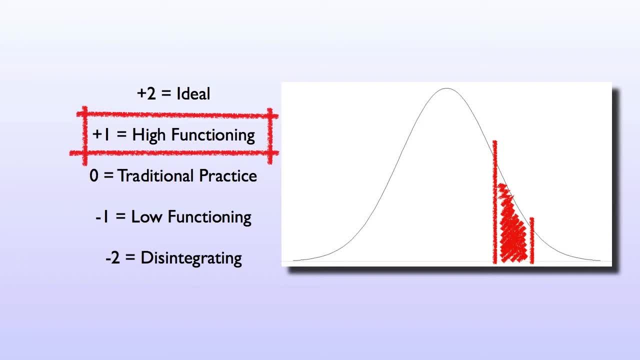 and work through differences on their own. They most often do this without the leader's help. The leader and members are learning to become genuinely vulnerable with one another, vulnerable on behalf of the team's inner sense of community and overall mission. In plus one teams, people, including the leader, show their vulnerability by openly acknowledging 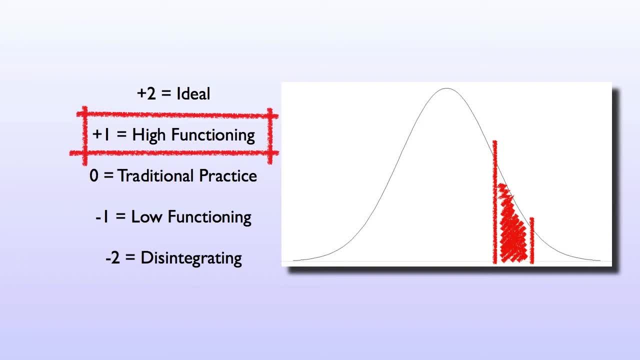 their mistakes in a group setting, asking for feedback, help and guidance from one another and by making sure that the team is doing what they're supposed to be doing. I'd emphasize that relationship building at the plus one level is conscious work. 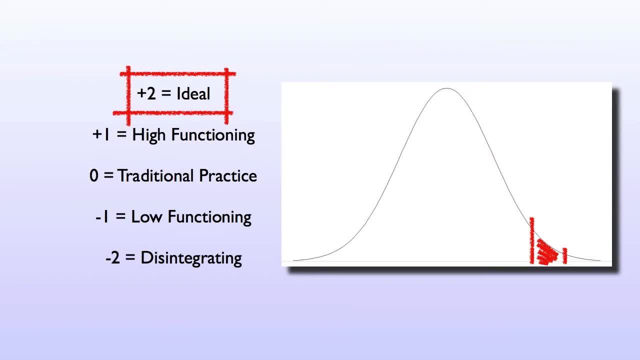 Above plus one are a few teams at plus two. They are great environments, but challenging ones as well. People at plus two- the ideal level- talk about anything in their team meetings, Few if any issues need to be addressed behind closed doors, If an individual's performance 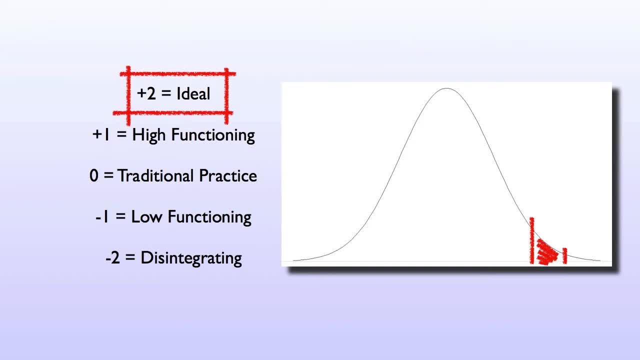 or interpersonal behavior is an issue, the group can and does bring it up to the team and talk about it constructively. Plus, two groups have gone beyond individual vulnerability to a point where defensiveness is rare, almost prohibited, as part of the group norms. These 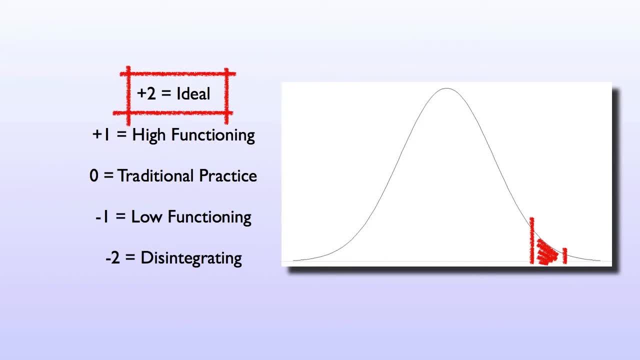 groups actively turn conflict into collaboration. The hallmark of such teams is their extraordinary sense of shared creative energy and interdependent purpose. The need for a central leader fades as each person exerts leadership within the group in a different way. Members feel deep support in their own life paths in a manner that goes beyond the bounds of any team or 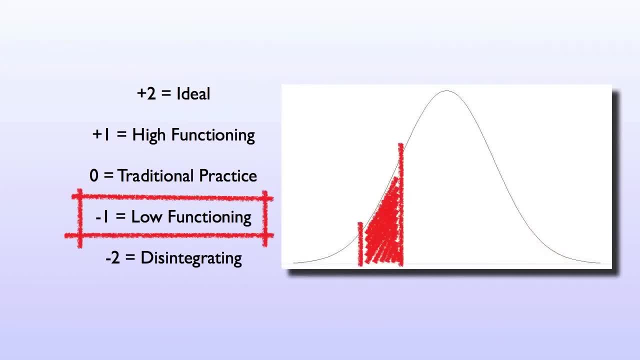 organization. On the other side of the coin are the minus one and minus two teams In minus one: low functioning groups. mistrust has taken hold. The group has internal fault lines and fracture points. Some would describe this level as a room full of broken glass where everyone 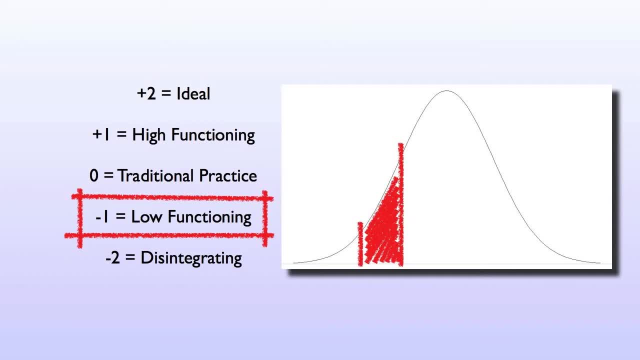 must step carefully. Typically, there are theories about why the group is the way it is, theories that are based in negative views of each other's motives or competencies. Minus one is often a cold war where misunderstandings and put downs leak onto the surface of team interactions. 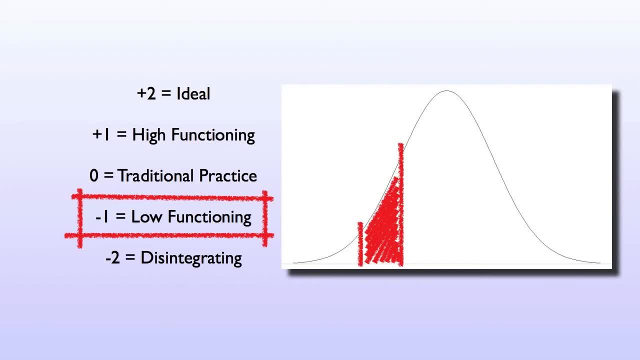 and there's talk, gossip and criticism in the background. Minus one is the land of undiscussables. Undiscussables are issues that people hesitate to bring forward to those who can do something about the problems because of their fears of negative repercussions or their sense that 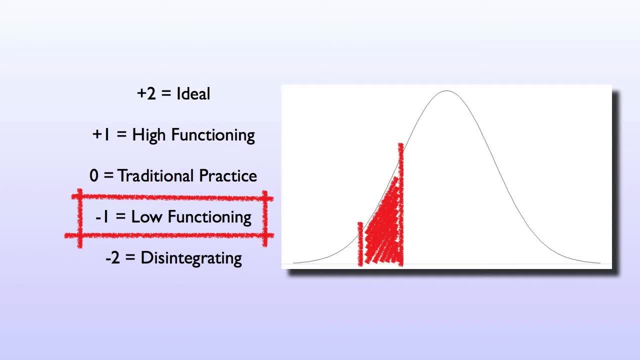 it won't do any good to try to address the issue issues. Often team members blame the leader for the group's problems, and they may or may not be right. Blame is a key word for minus one teams. Finding fault is always just around the corner. 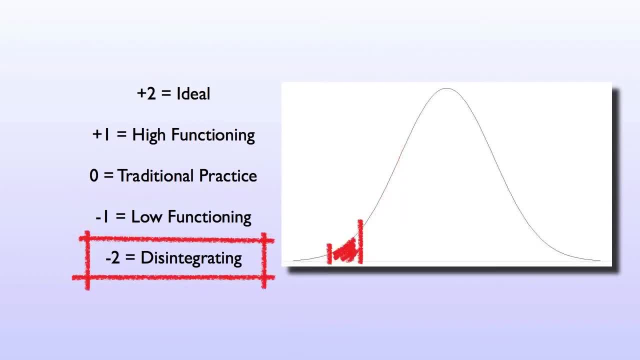 waiting to slip into the discussion. Finally, there are a few minus two teams. These are groups that genuinely deserve the label dysfunctional. The war that might have been cold in the past is now definitely hot and the team is disintegrating. Mistrust has become bound up. 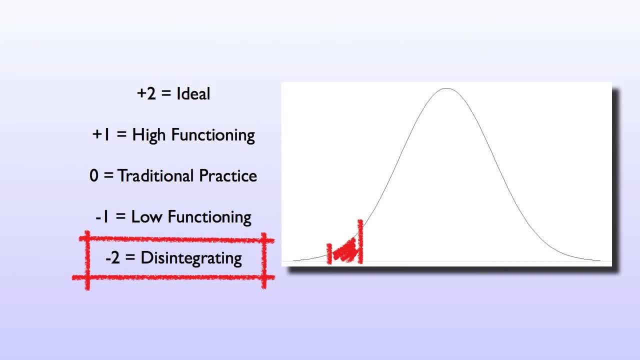 with anger, disappointment, a persistent sense of betrayal, and people assume that only by changing out team members or the leader will the problems be fixed. Many feel completely burned out by the conflicts. They may leave the organization just to get away from the disintegrating group. 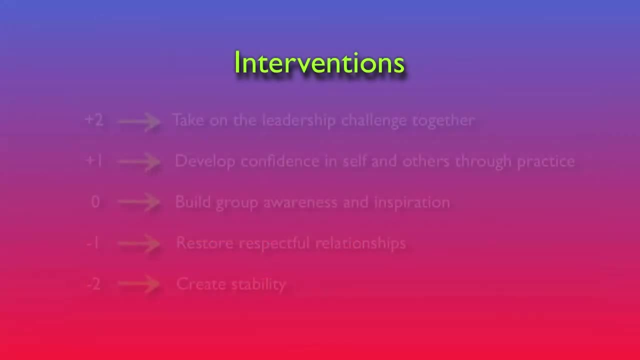 Once a group agrees generally on what level it is in the framework, it can then talk about what next. where do we go from here and how do we get there? In the survey document, this information is found in the intervention section and is fairly. 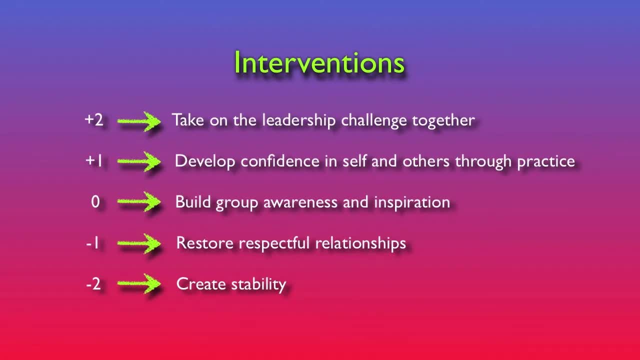 detailed. Please keep in mind, however, that the information in this section is not all-inclusive. Your group may need and want different things, so a thorough discussion is required. What I will share briefly now are the primary trust-building tasks for each level. They are: 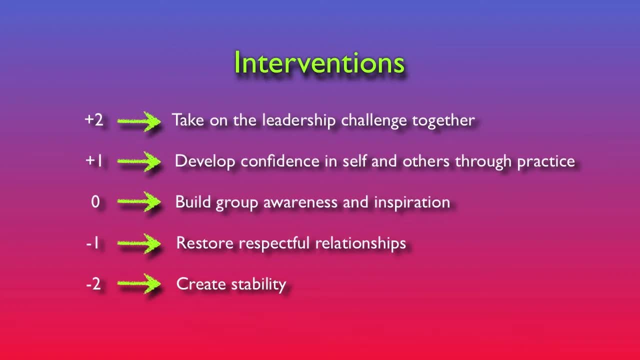 listed here and are general in nature. For levels minus two, minus one and zero. they focus two levels up, That is, two levels up. That is when a group is deciding what to do. it shouldn't just look at the next level and try to get. 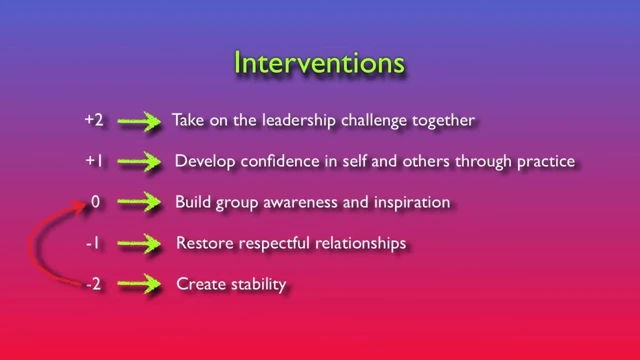 there, but instead look to the level beyond. If a group sees itself at minus two, it should look at the good sides of the null or zero level. If the team is at minus one plus one is an example of where it might aim to go. If the group is at zero, members can consider what there is to learn from. 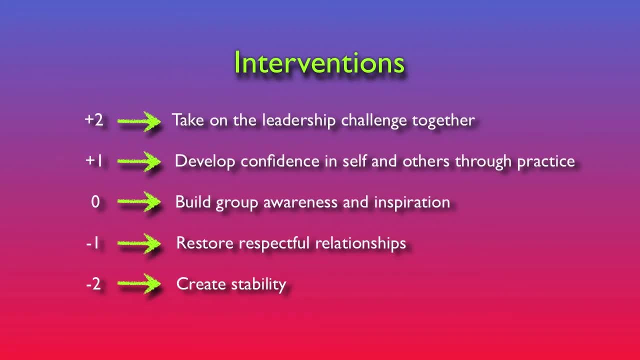 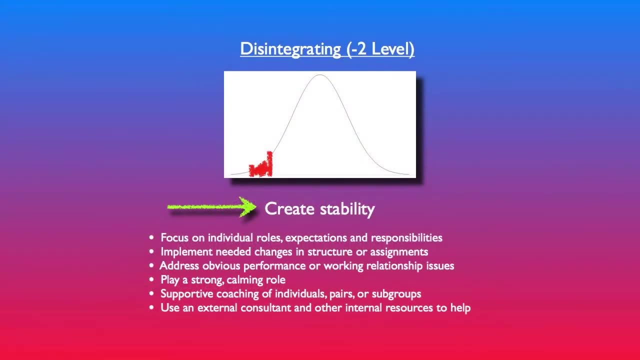 plus two. Let's look at these primary trust-building tasks for each level. I'll start with minus two and work toward plus two. If you rated your team as minus two, disintegrating, a primary thing that will aid trust is usually basic organizational stability. This is what 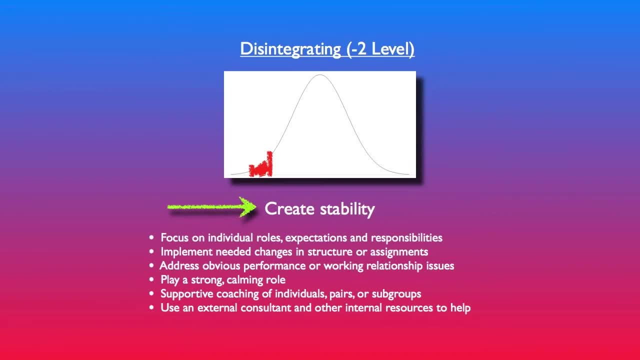 characterizes the null or zero level. people focused on their work and serving customers. So at minus two it usually helps to get clear about tasks, about individual and group expectations and roles. Stability means quickly and thoroughly addressing obvious performance or working relationship issues. 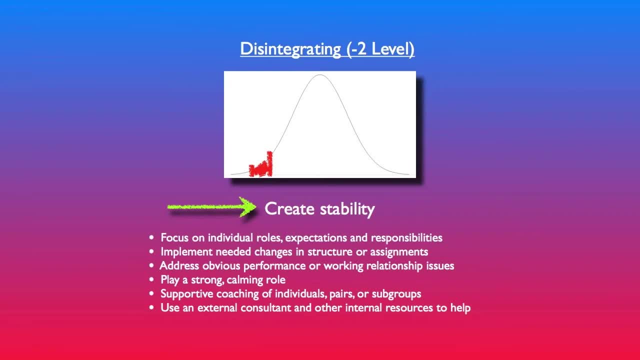 And these are usually right on the surface. They must be dealt with, even if it means that the team is reorganized or that some people go and some stay, including the leader. Small changes sometimes can mean a lot. It isn't always a big shift. The team will need help from outside, from an external, 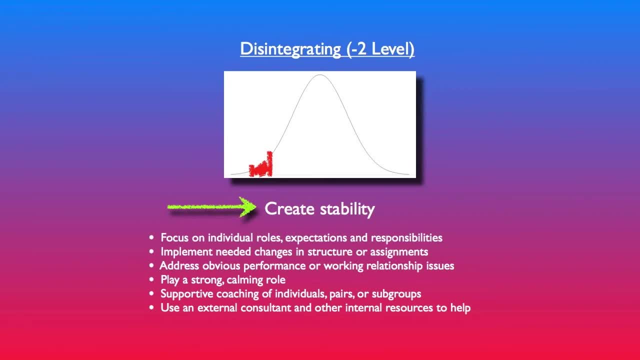 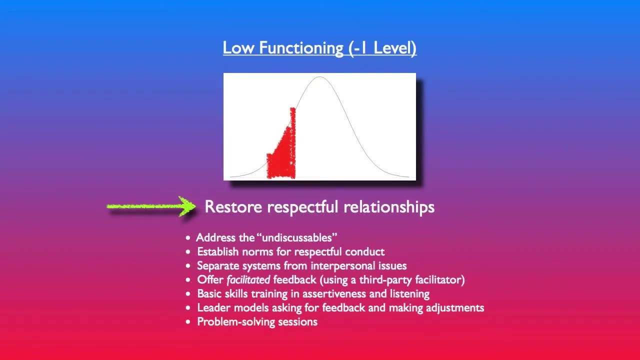 consultant or someone in human resources to advise and perhaps facilitate some of these tasks. If you rated your team as minus one, a primary trust-building effort is to make sure that the team is doing what they need to do. A major risk factor is restoring respectful relationships. work that. 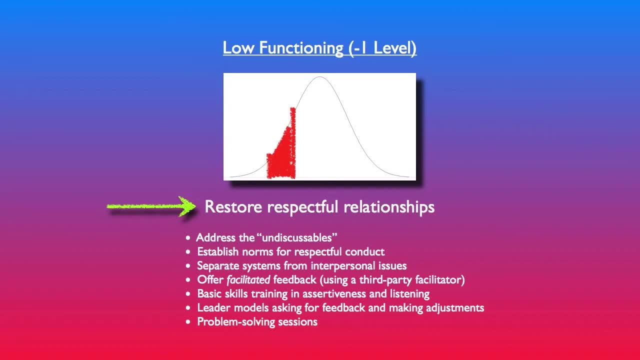 takes time, persistence and patience. Team members need to be encouraged to take risks again, to overcome the fear of repercussions or the sense that things can't change. What's undiscussable needs to come to the surface and be addressed in a facilitated way, And those who are leading must 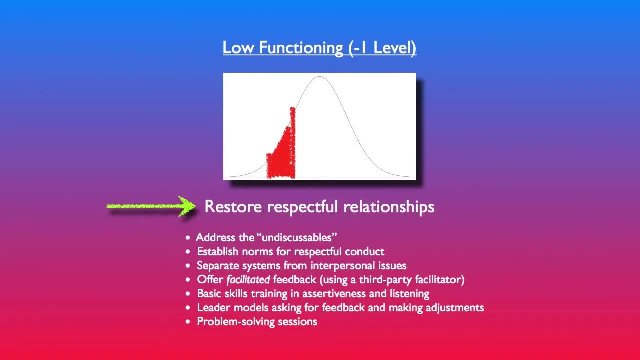 model the changes in their own behavior. first. When I say those who are leading, of course that includes the formal leader of the group, But it needs to also include those who are formal leaders as well, And that could be you. So whatever you can do to display what people do, 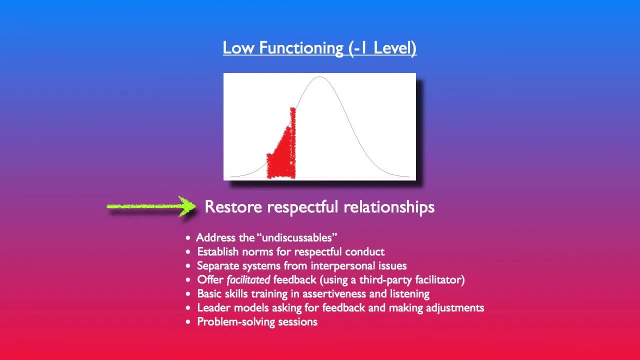 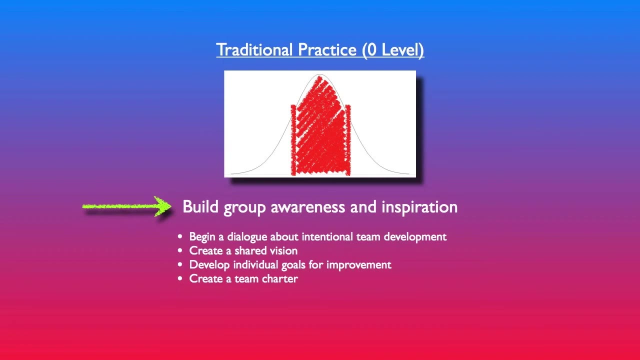 especially well at the plus one level, which is to take risks, ask for feedback and show that changes can be made safely if everyone pitches in is powerful and important work. The traditional practice level level zero is where most teams start The primary trust-building. 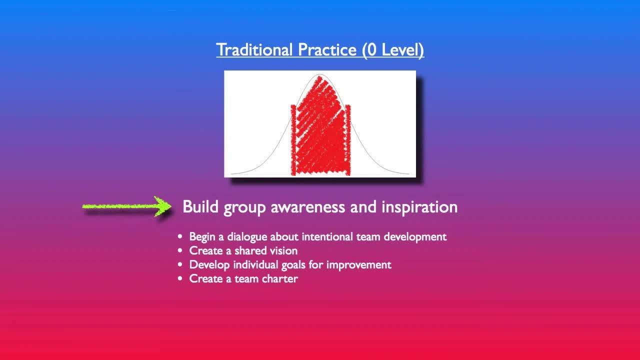 task is in helping foster a sense of group self-determination as a desired and conscious effort. People need to see why change might be important to them, why the risks to move higher on the trust continuum could be worth it. The first step may be helping people notice that the group could be and 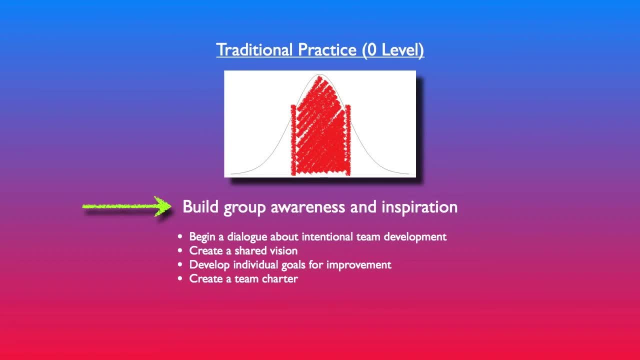 really needs to be more than the sum of its parts. The group has combined power and combined potential that it will realize only if people choose to go in that direction. That power and potential are based in the decisions members make together, the processes they use to get things done collaboratively. 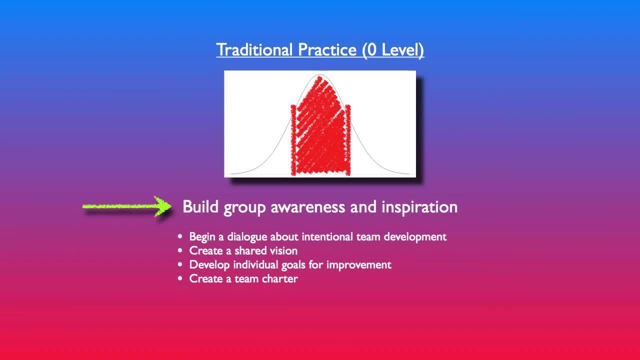 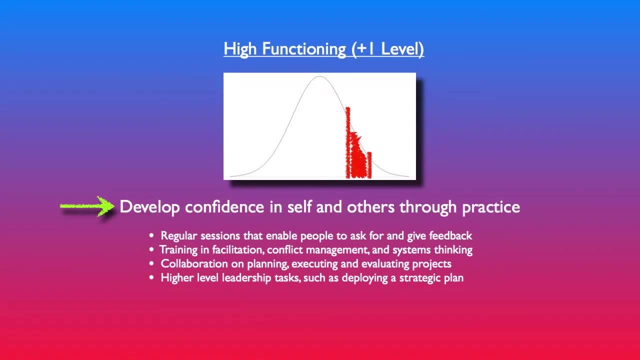 and the decisions they make together And the work they mutually do to improve the quality of their relationships. For high-functioning plus one teams, the primary task is to overcome the anxiety people hold about getting real with one another. This is the most misunderstood of the levels It 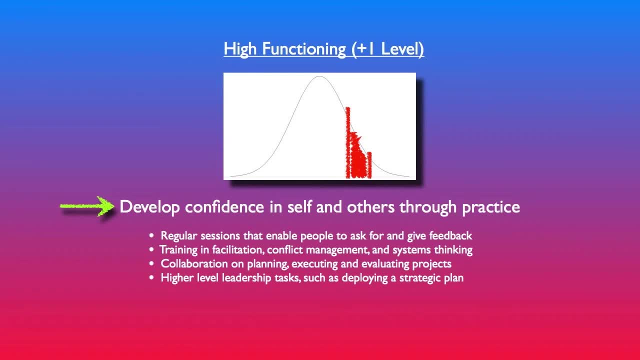 isn't about creating harmony, but it's not about intentionally creating conflicts or being abrasive with each other either. It is about choosing to open up the opportunities for personal growth in a combined way. Sometimes that's scary work because people worry it will mean confronting other members. 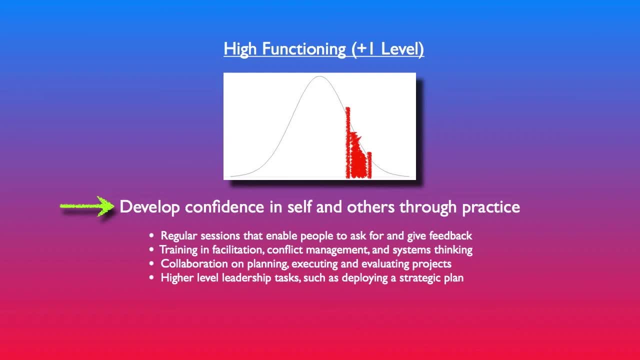 banging people around with negative feedback or maybe hurting others on the way to the truth. In my experience, that's not the real work. It's the feared work. The real work is in taking the risk to develop and grow as a human being and professional in front of and with other people. 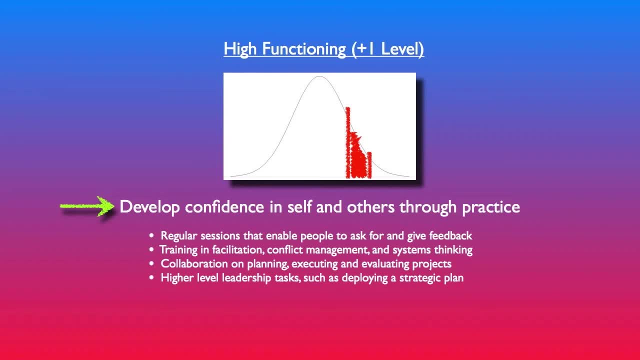 Plus one is about enhancing personal capacity for disclosure, about supporting each other especially well, while each person gradually learns how to ask for feedback, confront themselves, not others, and learn to make the changes that feed their own maturity and wisdom. For ideal, plus two teams, the primary task is really one of constantly exercising new. 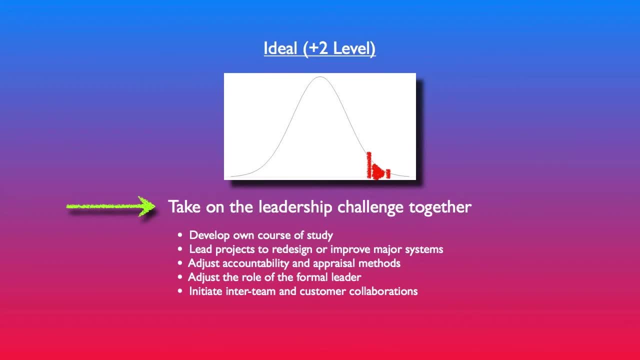 capabilities by taking on the leadership challenge together. This challenge is about the increasingly frequent replacement of a central leader figure with a group's own combined leadership capacity. Ideal teams exercise this capacity by learning to collaboratively change systems, change the organization, change products, change programs. They are creative and strategic innovators. 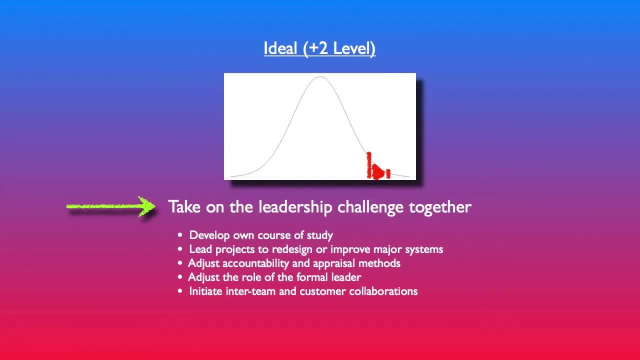 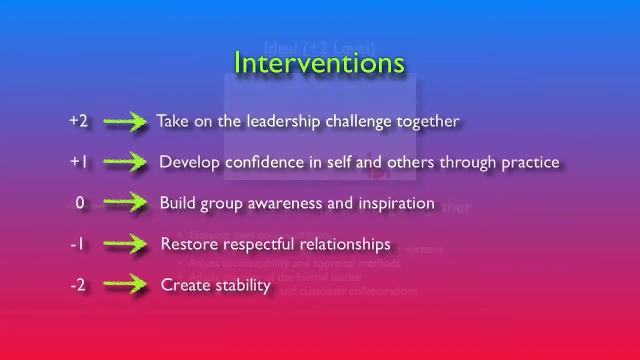 a powerhouse team, So their work is in deciding together what's most strategic and big enough to work on, and going after it in a highly resourceful way. Additionally, the team can also be challenged to come up with its own self-appraisal and combined group reward mechanisms. 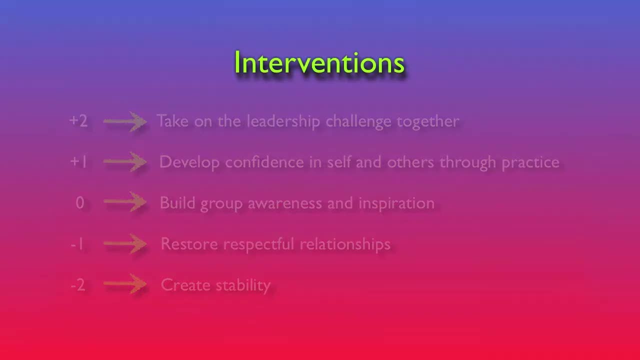 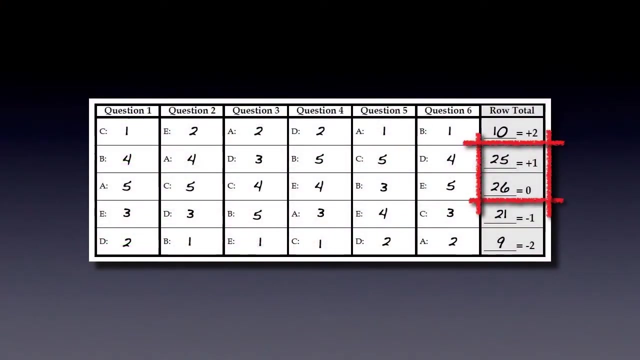 As a final part of this tutorial, I want to identify another important way team members can use their score sheets to think about what they might do together to enhance trust. This is likely to be particularly helpful where the team's behavior seems to cross over more than one level. Take a look at this score sheet. In the row total column, you can see 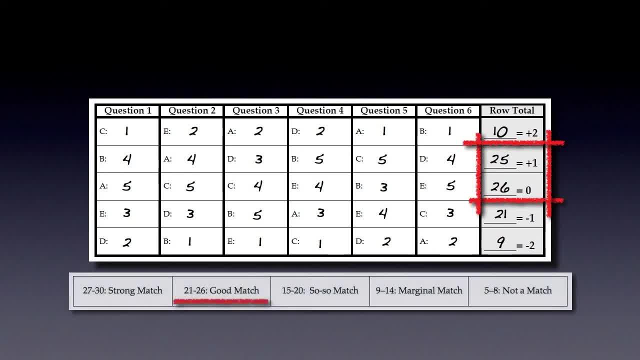 that the scores for the zero and plus one levels are almost identical. To get to where a team might improve, first take a look to see if the highest numbers fall in the good to strong match range. If they are spread out so that the row totals get down into the 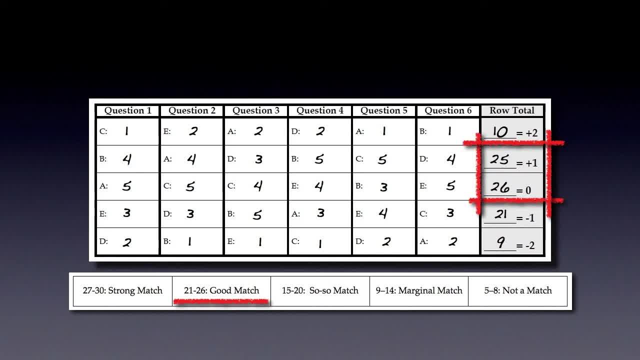 so-so match range, then you might want to go back and look very carefully at what's happening on your score sheet. Go back and take a look at the questions and how you answered them. What's causing the numbers to be so dispersed? Assuming, however, the numbers are in the good to strong match range, but at more than one?